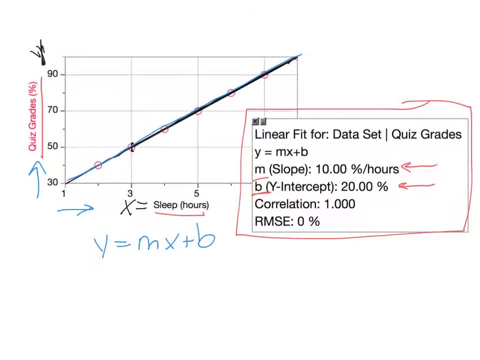 line and all you have to do really is just literally copy and paste the Y that we have with Y in the equation, the X with the X in equation, our slope here and B here with the B in the slope in our equation. so let's do that, so our Y is quiz grades. 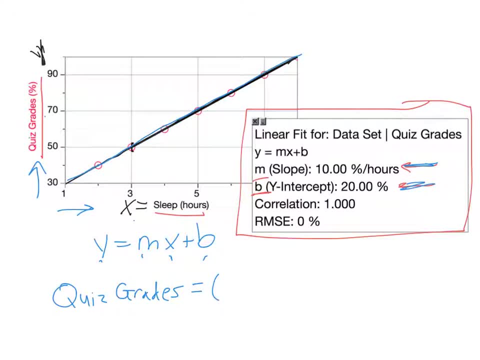 equals our M, and here our M is 10% over hours and our X is the sleep, and our B, like it says here on our graph, on our linear fit box, is 20%. okay, and that's it all right, but what's most important? well, in addition, 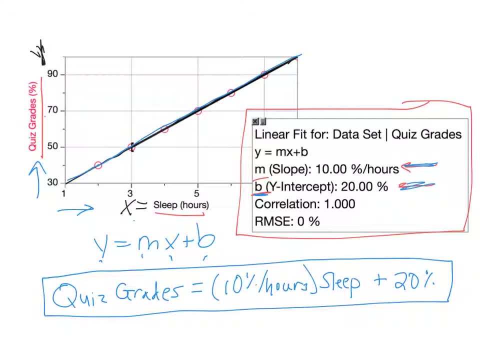 to being able to do this. it's also important to understand what this equation is telling us. okay, it relates sleep to your quiz grades, so your X is related to your Y. how well, it tells you that for every one hour of sleep, you get 10%. okay, that's what we call for: every statement, for every 10%. 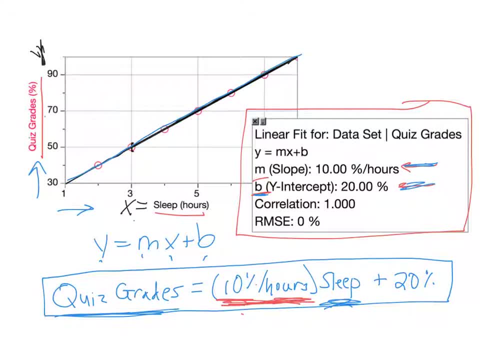 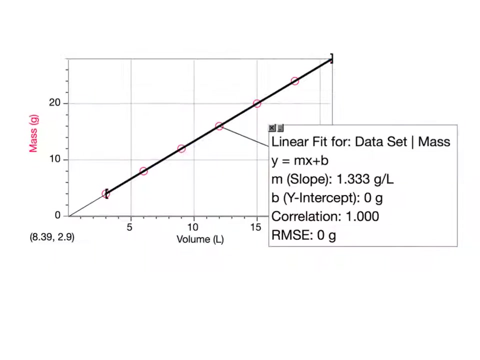 there are one hour of sleep or you can flip it. for every one hour of sleep there is 10%. okay, what the y-intercept tells us is how much percent you get when the sleep or the X variable is zero. okay, let's take a look at the next graph. all right. next example: we've got mass, first volume here. 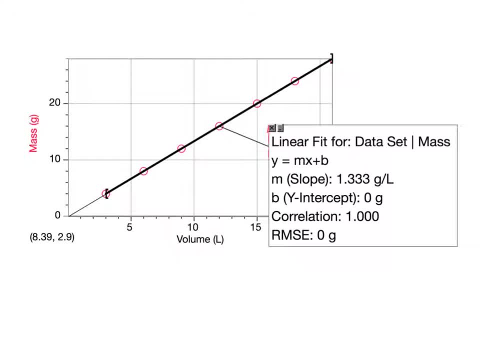 okay, let's try to give this a shot. we've got our box here, you've got our slope and we've got our y-intercept B. okay, we've also got our X variable, which is volume, and our Y is our mass. and so let's begin. Y equals mx plus B. okay, so what's our y? looks like we've got masses. our y.